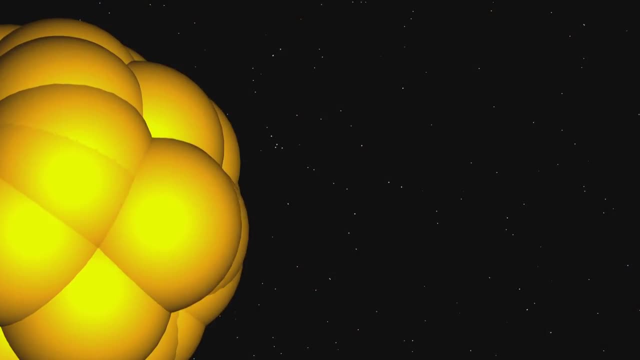 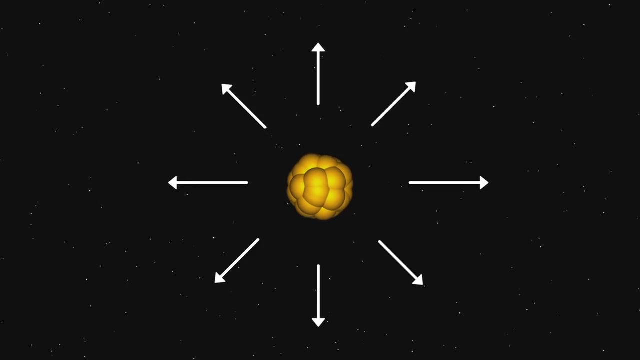 all packed together in a ridiculously tiny volume, And a proton on the surface is repelled with a force of just over 70 pounds. So if these protons are all getting pushed apart from one another, what keeps them together? There's only one possibility: There has to be a force that is even stronger, that counteracts. 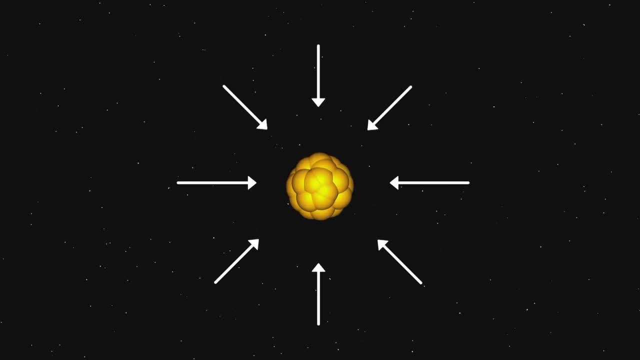 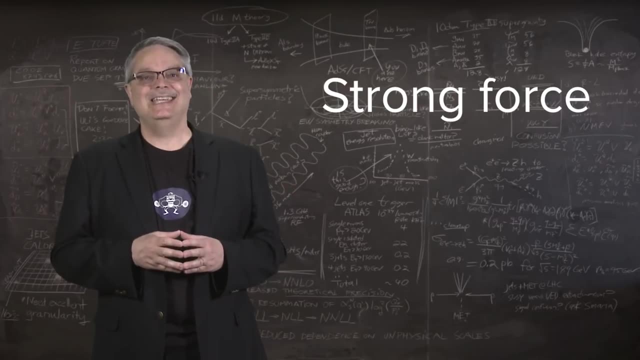 the electromagnetic repulsion, And the name for that force is- you got it- the strong force. What do we know about the strong force? Well, we know that it's strong And it can't just be a little stronger than the electromagnetic force. That's because if the two forces 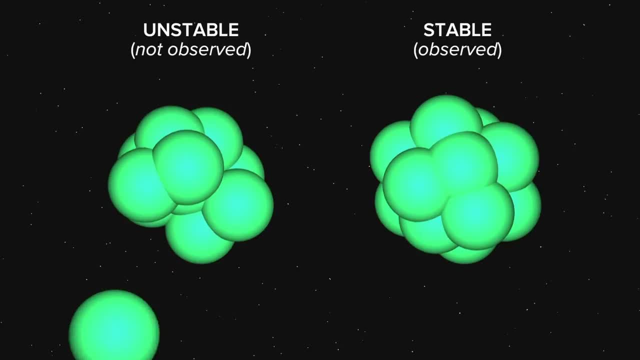 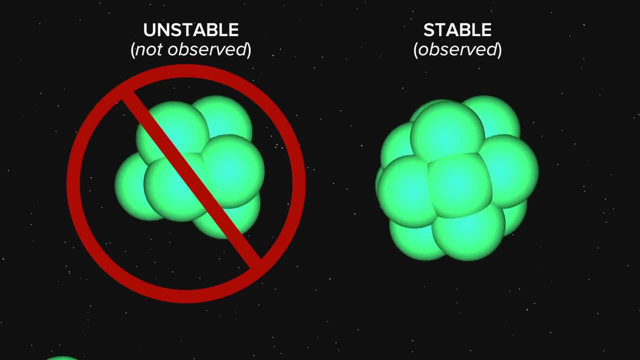 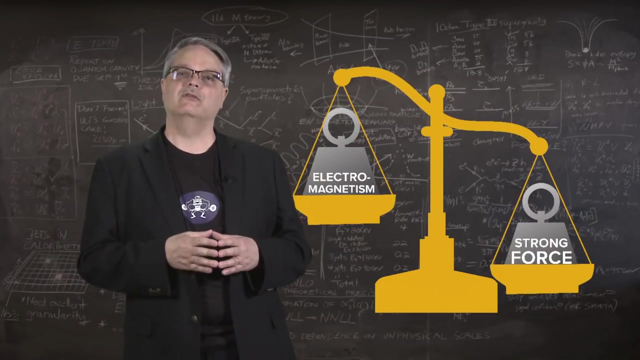 were pretty similar, it would be easy to knock protons out of the nucleus of atoms. And we know that's not true, because nuclei last for millions and even billions of years. So the strong force has to be way stronger. From tests we know that the strong force is about 100 times stronger than the electromagnetic. 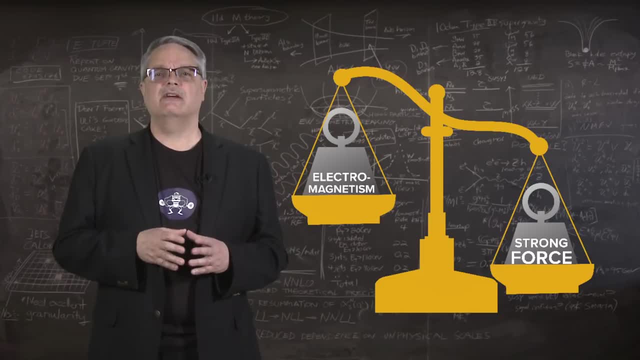 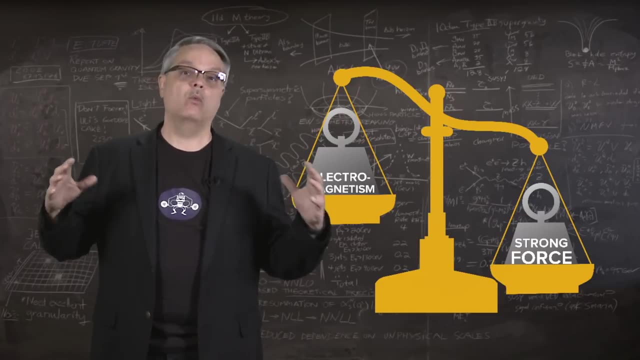 force. But the story is a bit trickier than that. After all, if the force is so high, what keeps the strong force from continuing to gather protons until the whole universe consists of one big nucleus? If we look at the periodic table, we see that the highest stable element has no more than 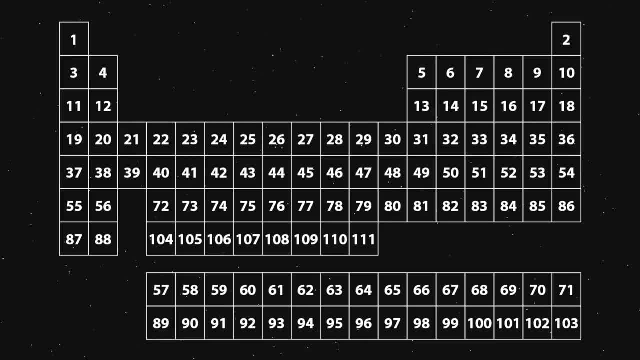 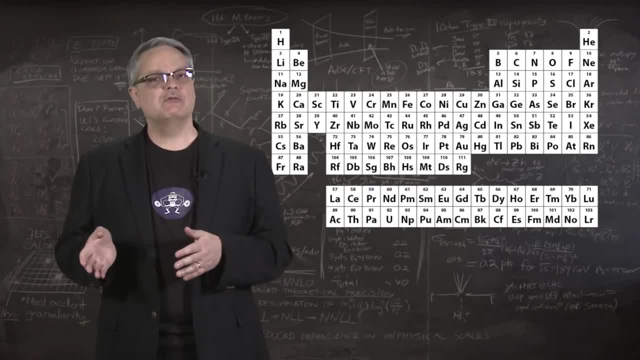 about 100 protons in it, And yes, I know that the nuclei also contains neutrons. That doesn't change much in what we're talking about here. So it seems that with more than about 100 protons, the strong force can't hold it all. 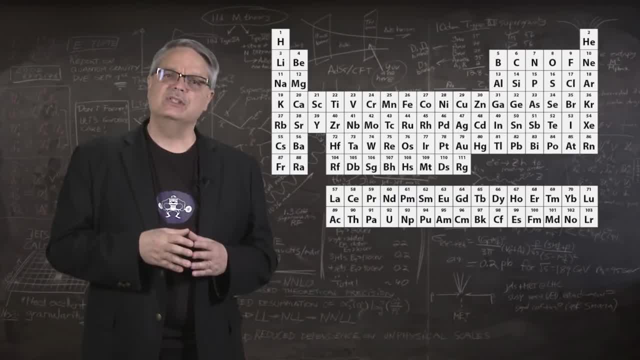 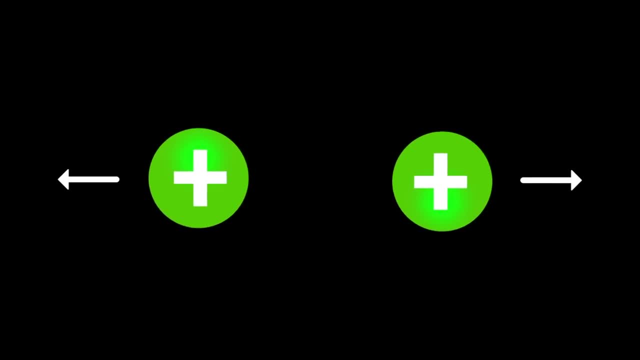 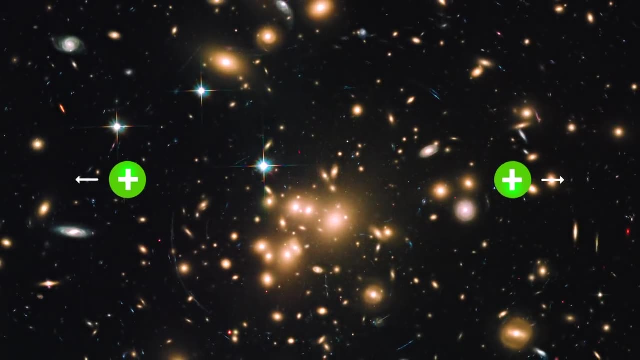 together. What's that all about? It turns out that there is a property of the strong force that is quite different than the electromagnetic force. Electromagnetism has an infinite range. In principle, two electrically charged particles will feel a force between them if they're separated by the entire universe. Okay, the 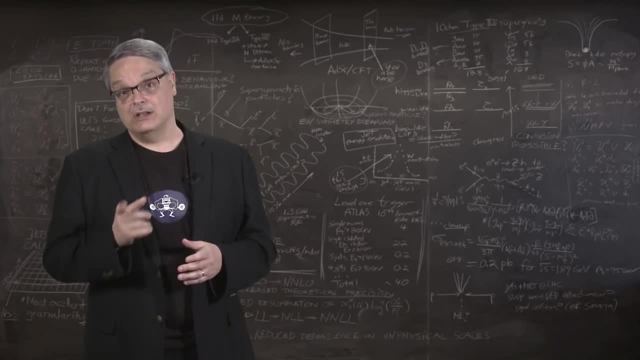 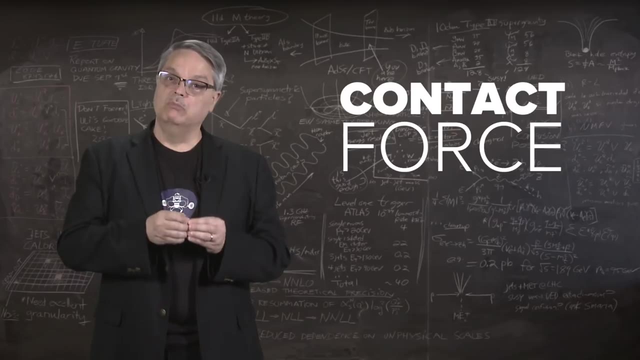 force would be small, but in principle it's true. In contrast, the strong force is more like a contact force. When two protons touch each other, they feel the strong force. Pull them apart a little bit, they feel the strong force. 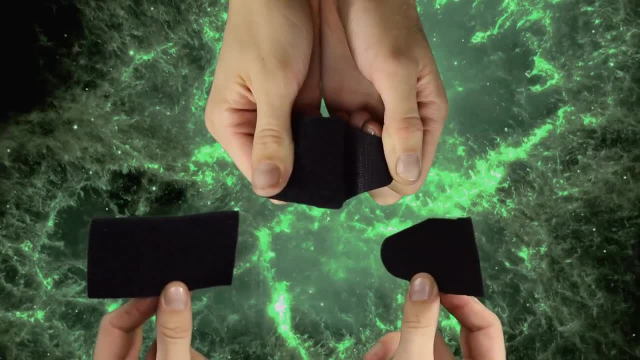 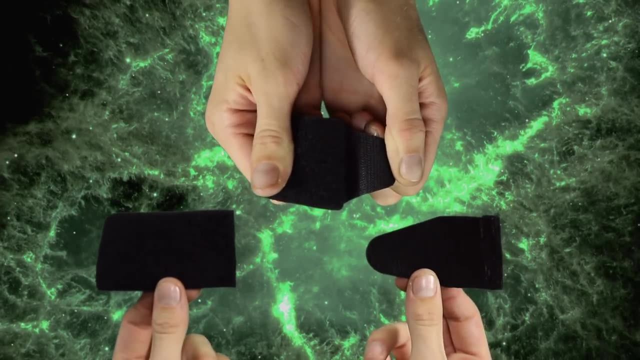 And in that way the strong force goes to zero. In a way, the strong force is a little like Velcro: When two pieces of Velcro aren't touching, the two pieces feel no force toward one another. So that's the strong force. It is stronger than the electromagnetic force, but it has